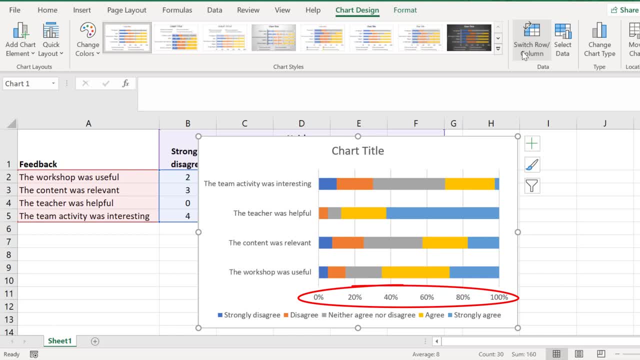 Looking at each bar, you can easily see that they total up to 100% percent. however, it's hard to know what the value is for each response, so let's add some data labels to the graph. with the graph selected, go to add chart element data labels. then select a suitable. 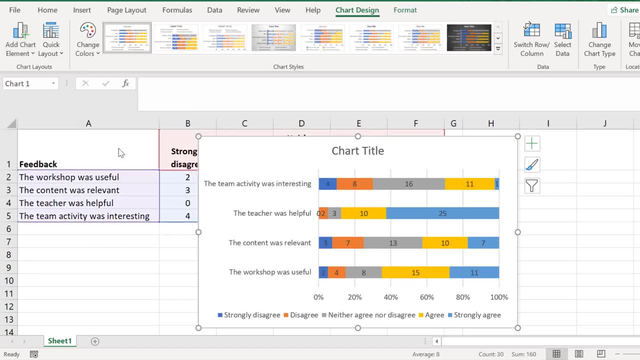 location. i like to use the center option now. as you can see, the number of responses in each cell are included in each color response block, so i can easily see that eight students disagreed that the team activity was interesting, for example, instead of showing the number of responses in each cell. 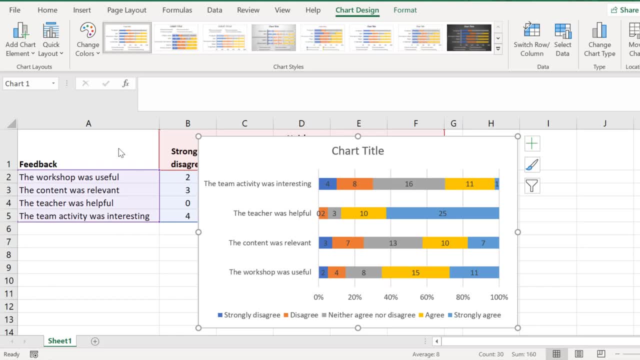 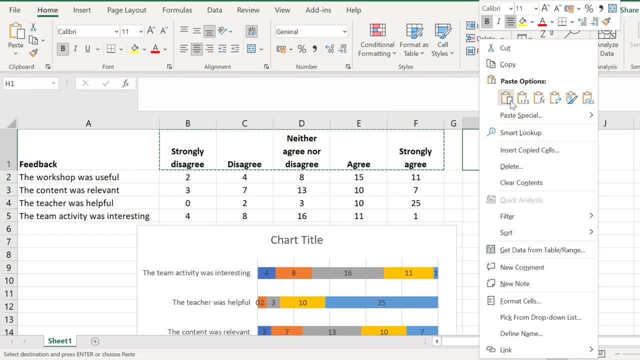 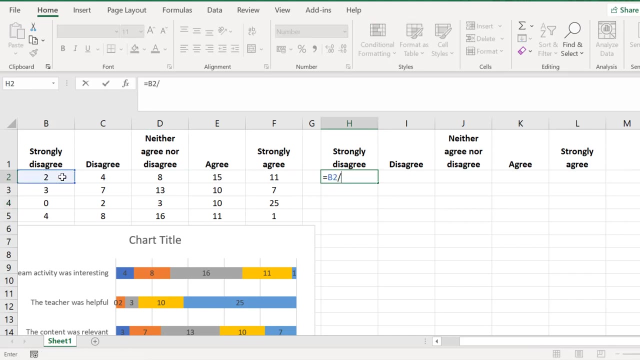 i could show the percentage value instead. to be able to do this, i need to work out the percentages of each response for each question. to do this i'll copy my response headers, then in my first cell i will enter equals. then i'll select my first cell, then i'll divide by the total number of responses. 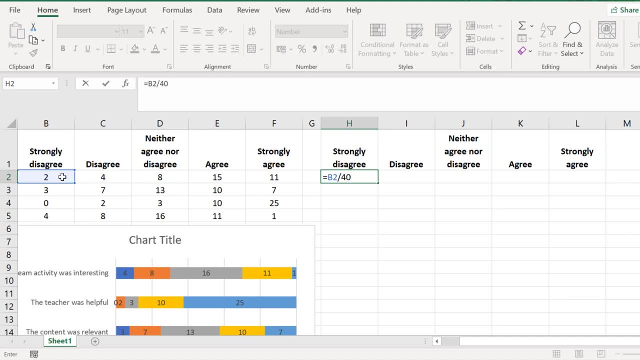 i had, which is 40 in this example, then i'll press the enter key. i now need to do this for all of my cells. to do this, i can use excel's autocomplete feature. with the first cell selected, i'll use the little green square to drag the formula down. then I would drag it across. 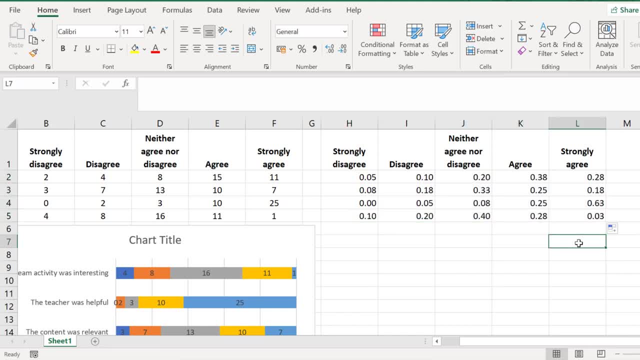 The next thing I must do is to change the format of these cells to a percentage. So with all the cells selected, I will go to home. then in the number section here, I will use the drop down menu to change the cell format to a percentage. 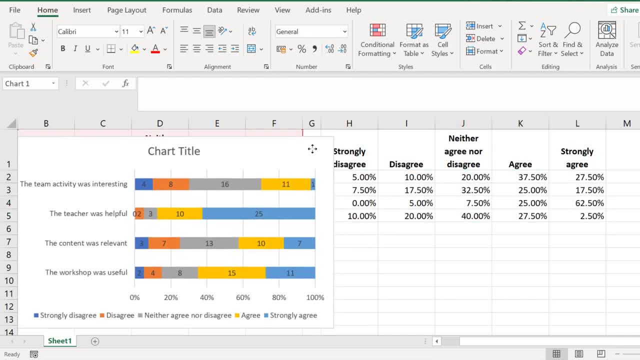 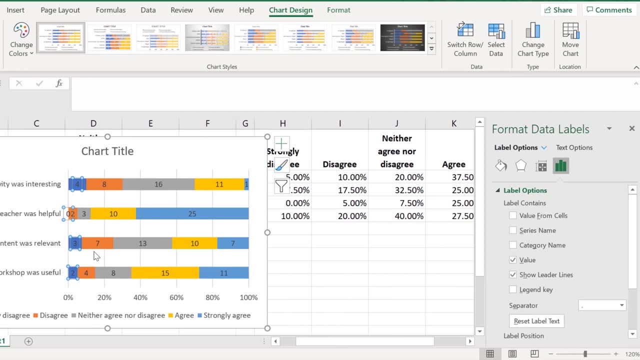 To be able to add this as a data label. I will select my graph, then I will go to add chart element: data labels- more data label options. A new sidebar should open to the right. I will select the label options icon to the right and then click the label options header. 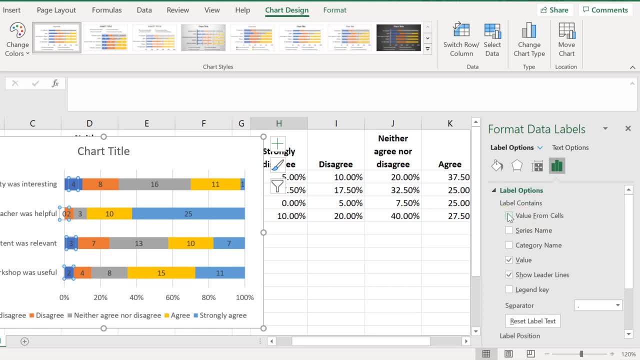 Then I'll select the value from cells option. Now I need to select the cells containing the percentage values from my first column, which is the strongly disagree response. Once done, I'll press the enter key on my keyboard to add this to my chart. 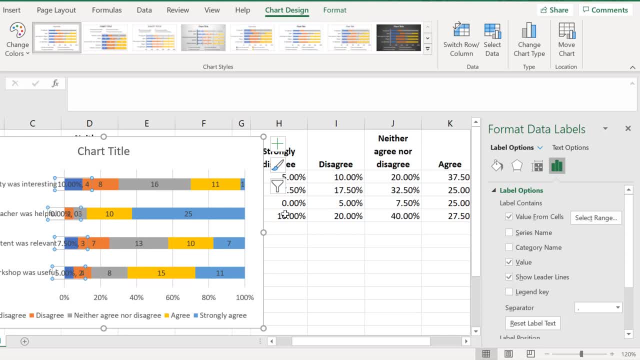 It looks slightly messy at the minute, and that's because the actual response value is also being shown alongside the percentage value. To remove this, I will simply deselect the value option here. Now, only the percentage value is being shown. What I need to do now is repeat this process, but for the other response columns on my graph.